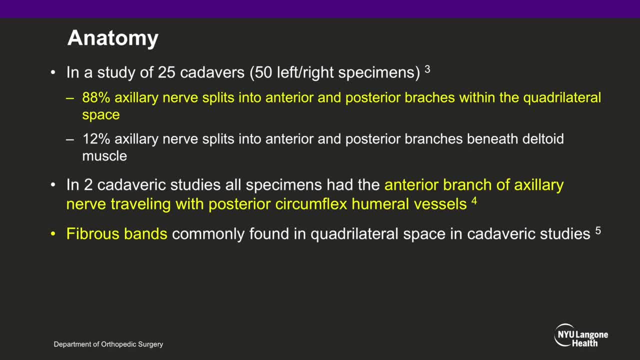 In a study of 25 cadavers, 88% of specimens were found to have an axillary nerve that splits into anterior and posterior branches within the quadrilateral space, 12% of specimens were found to have an axillary nerve that splits into anterior and posterior. 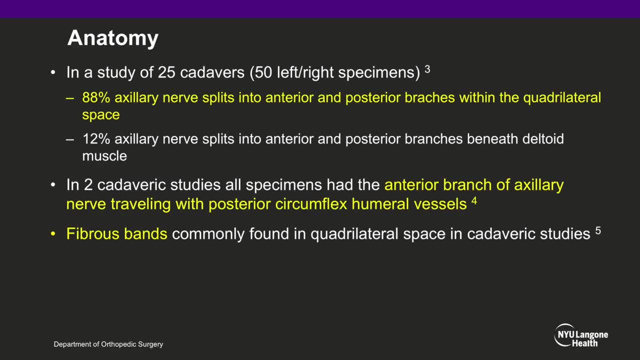 branches within the deltoid muscle. In two cadaveric studies, all specimens had the anterior branch of the posterior nerve traveling along with the posterior circumflex humeral vessels. Fibrous bands are also commonly found in the quadrilateral space of cadaveric specimens. 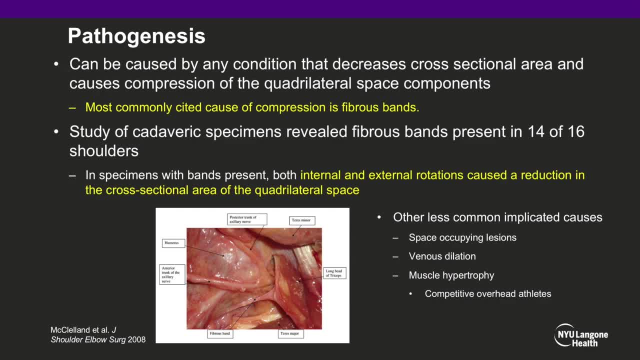 Quadrilateral space compression syndrome can be caused by any condition that decreases cross-sectional area and results in a compression of the quadrilateral space components. One of the most commonly cited cause of compression is fibrous bands. In a cadaver study, it was revealed that fibrous bands were present in 14 of 16 shoulders. 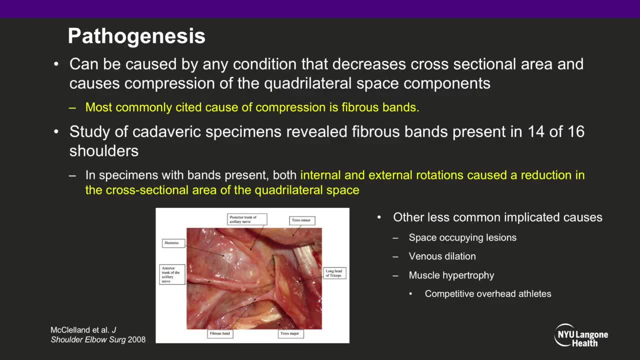 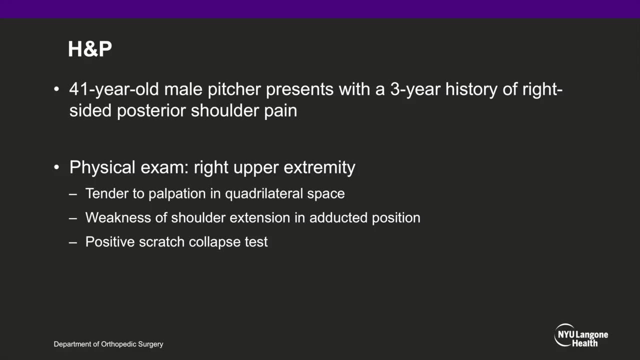 In specimens with bands present, both internal and external rotations caused a reduction in the cross-sectional area of the quadrilateral space. Other potential causes that are less commonly implicated include space-occupying lesions, venous dilation and muscle hypertrophy. The patient in this case is a 41-year-old male pitcher in a baseball league. 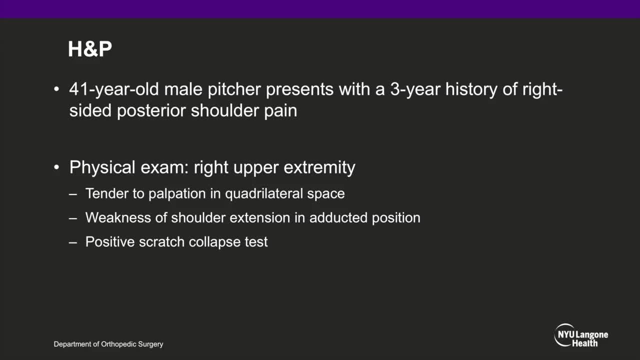 He presented with a three-year history of right-sided posterior shoulder pain. He was tender to palpation in the quadrilateral space and exhibited weakness of shoulder extension in the adducted position. Preoperative examination demonstrated a positive scratch collapse test which aids in the diagnosis of quadrilateral space syndrome. Here the surgeon is testing. 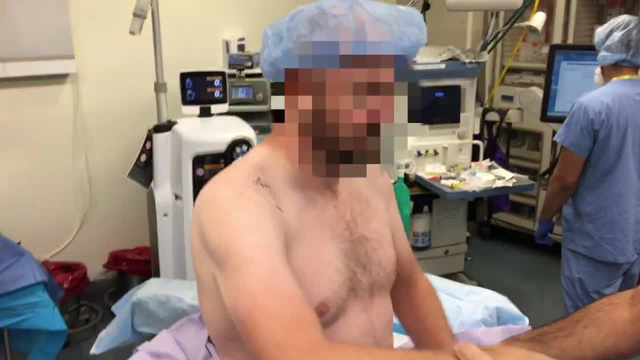 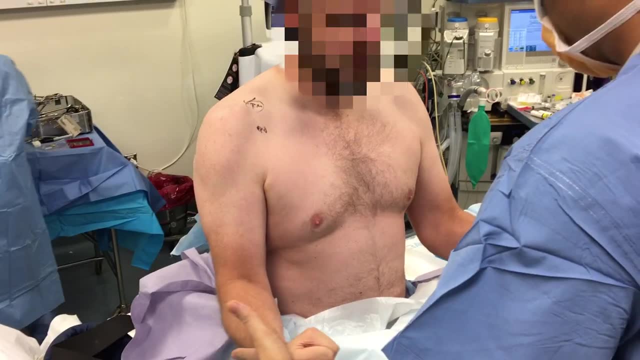 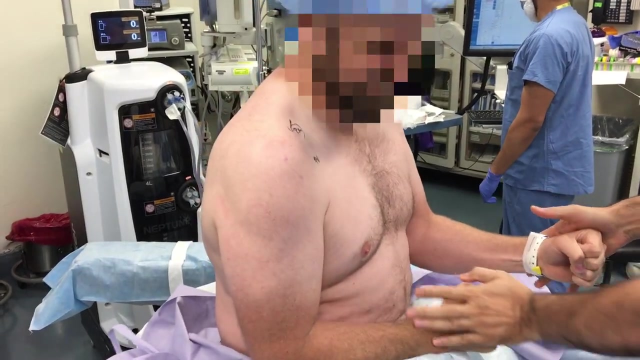 shoulder extension and external rotation against resistance. before and after stroking the skin in the axillary nerve distribution, Stimulation of the sensory pathway leads to a temporary tonic and inhibition of the posterior deltoid and teres minor, resulting in weakness in shoulder extension and external rotation. A right upper extremity angiography. 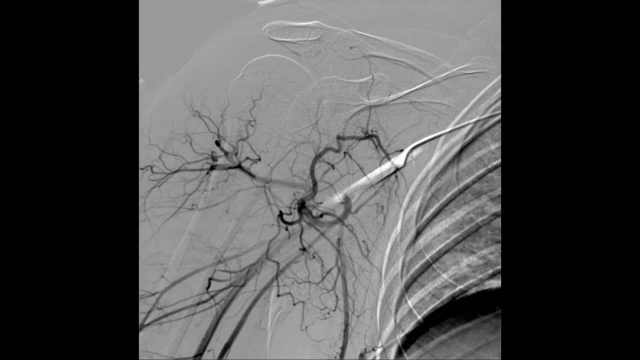 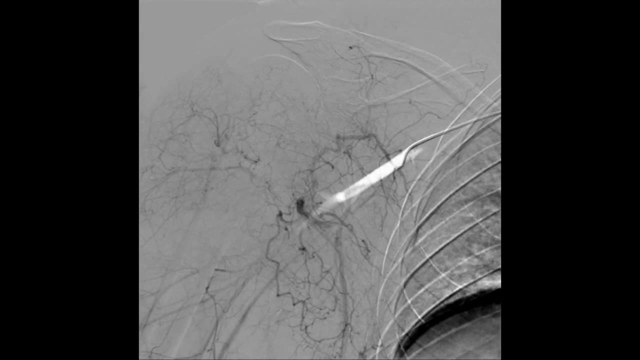 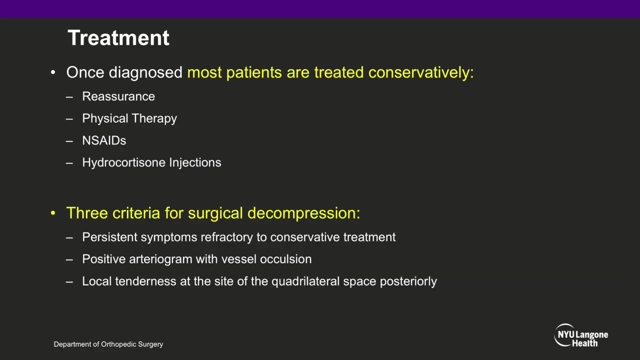 displays abrupt occlusion of the posterior humeral circumflex artery within the quadrilateral space with dynamic maneuvers of the right shoulder. An MRI of the shoulder also demonstrated a posterior labral tear. Once diagnosed, most patients with quadrilateral space compression syndrome are treated conservatively. 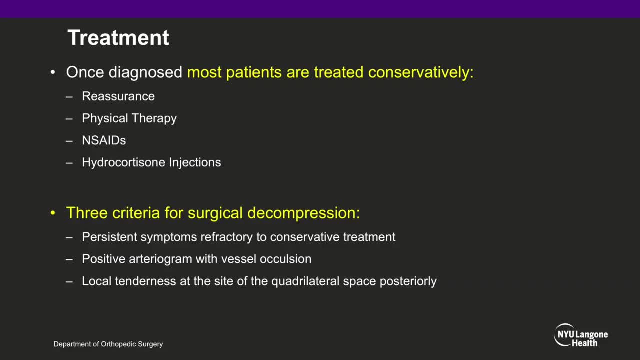 With reassurance: physical therapy, non-steroidal anti-inflammatory medication and hydrocortisone injections. Three criteria commonly cited for surgical decompression include persistent symptoms refractory to conservative treatment, a positive arteriogram with vessel occlusion and local tenderness at the site of the quadrilateral space posteriorly. 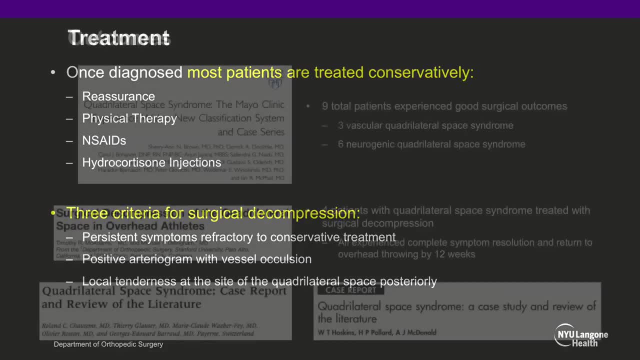 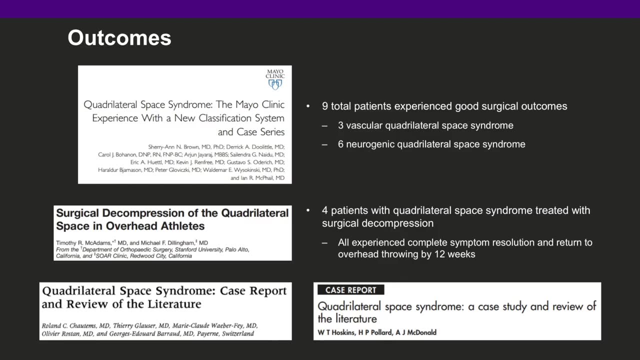 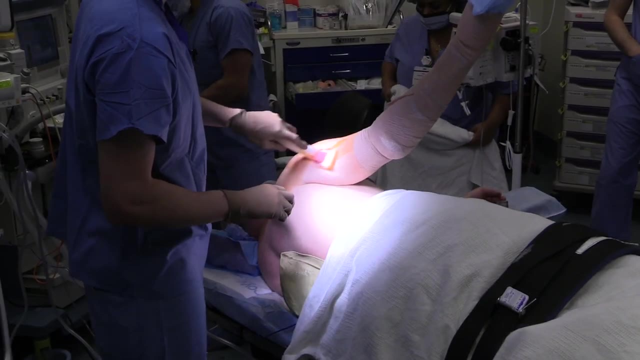 In this case, our patient exhibited all three of these criteria. Although limited to mainly small case series and case reports, literature on outcomes following surgical decompression is very promising. with complete or near complete symptom resolution, The patient is positioned in the lateral decuba disposition. 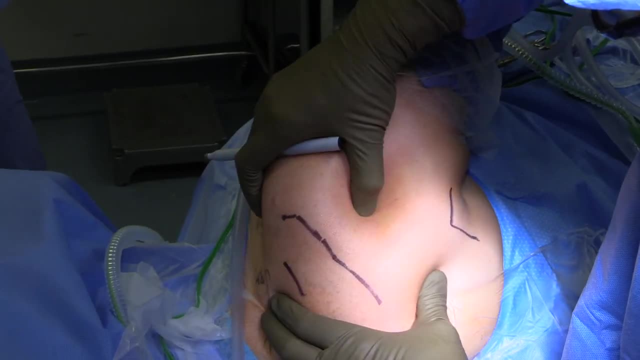 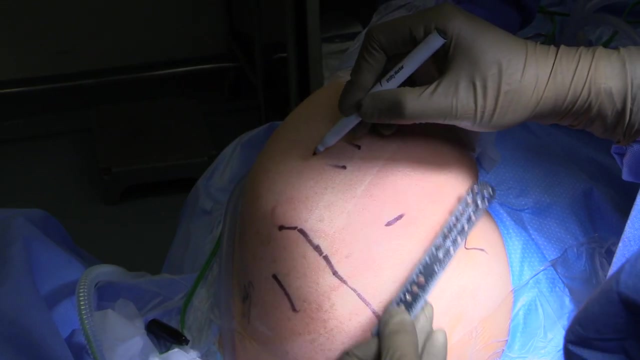 Anatomic landmarks are identified, including the posterior lateral corner of the acromion, posterior axillary fold and the tract of the axillary nerve which is approximately seven centimeters distal to the posterior lateral corner of the acromion, In this case, arthroscopy portals. 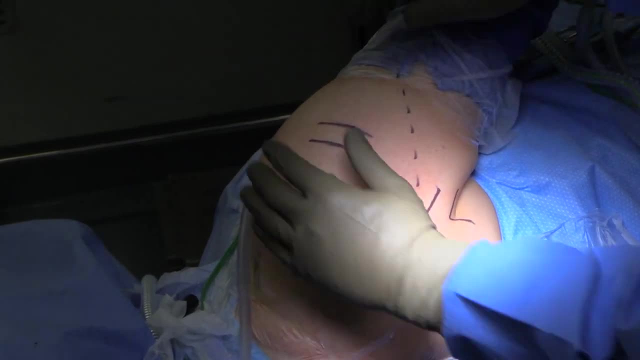 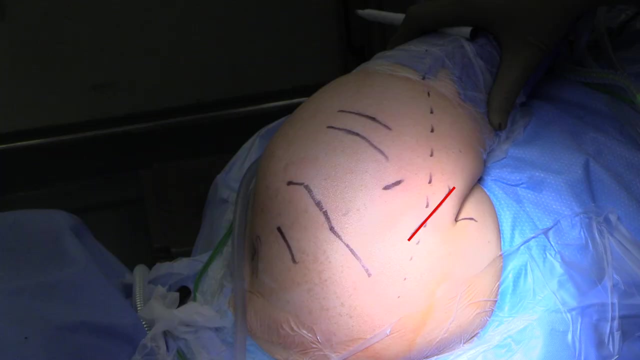 are also marked for surgical treatment of his labral tear. The dashed line represents the posterior border of the deltoid and a five centimeter incision is made relatively parallel to this line, but slightly medial, in order to access the axillary nerve, the teres major and the quadrilateral space. This is in contrast to the classic posterior. approach to the shoulder with a deltoid split utilizing an incision from the posterior lateral corner of the acromion to the axillary fold. This technique can still be used, depending on surgeon preference. However, for this release, we prefer this incision in lieu of the incision. 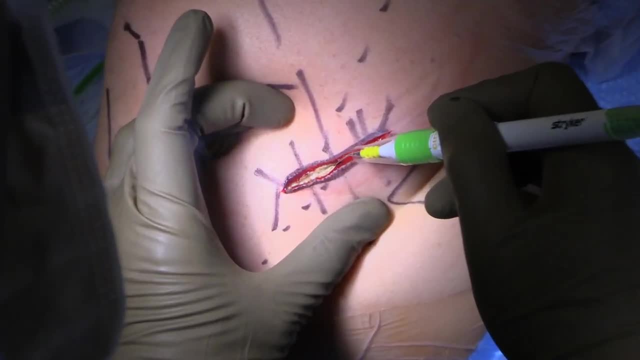 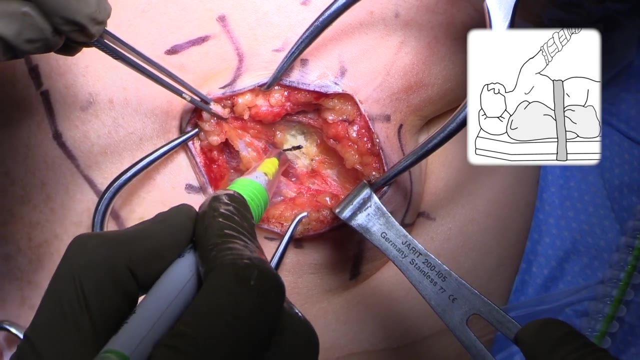 In this view, we've zoomed into the surgical field. The patient's head is to the left and the hand is to the right. Following the incision, subcutaneous dissection is performed with a needle tip, bovie, to expose the first layer, which is the deltoid, Full thickness subcutaneous flaps. 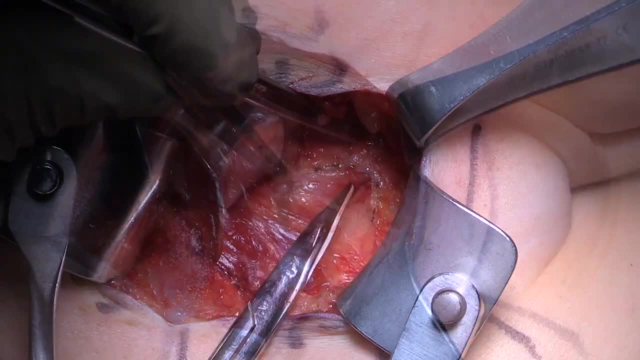 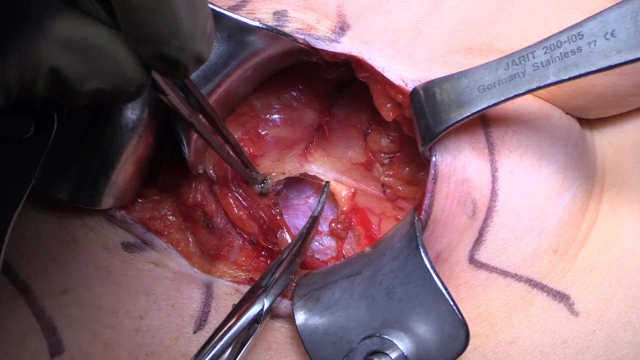 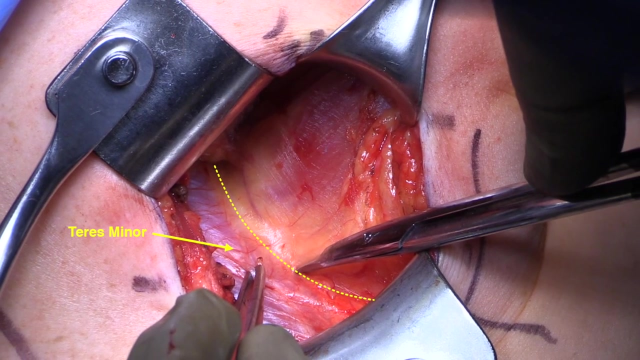 are elevated. The posterior border of the deltoid is then elevated and retracted anteriorly to expose the second layer, allowing visualization of the teres minor, teres major and posterior lateral Long head of the triceps. The inferior border of the teres minor is identified and exposed The thick fascial 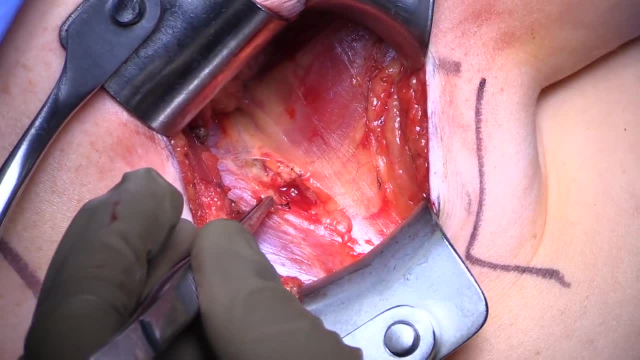 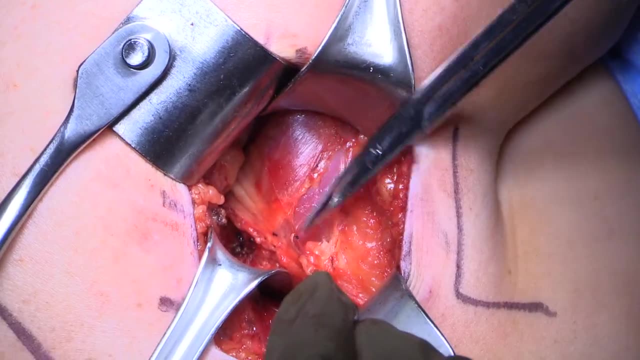 band of the inferior border of the teres minor is released to identify the nerve to the teres minor. Meticulous dissection is required at this stage because of frequent bleeders. The nerve to the teres minor is then traced back to the main trunk and posterior and anterior 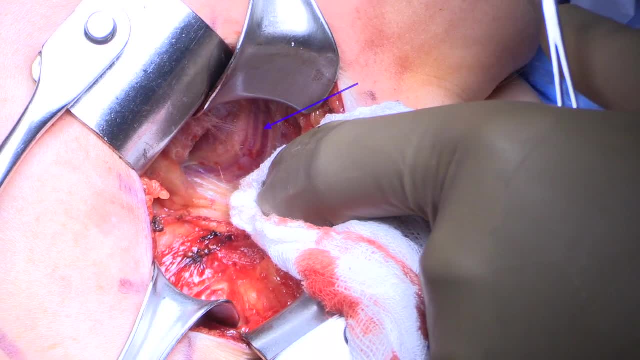 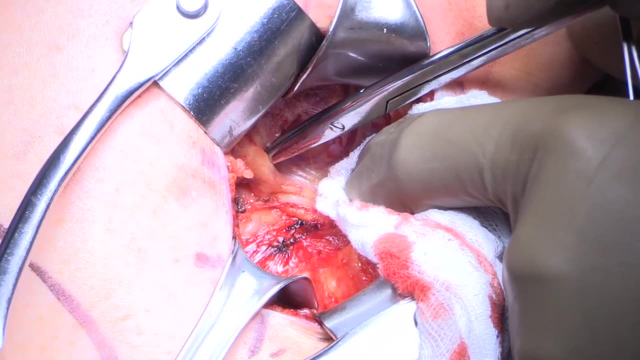 divisions of the axillary nerve. The posterior circumflex humeral vessels can now be visualized. The posterior divisions of the anterior and anterior divisions of the posterior and anterior division of the axillary nerve is identified and a vessel loop is passed around the axillary nerve. 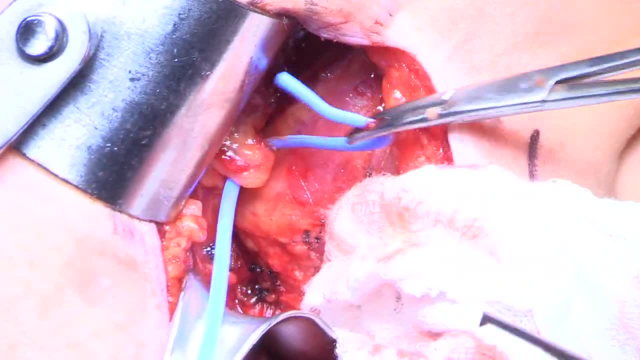 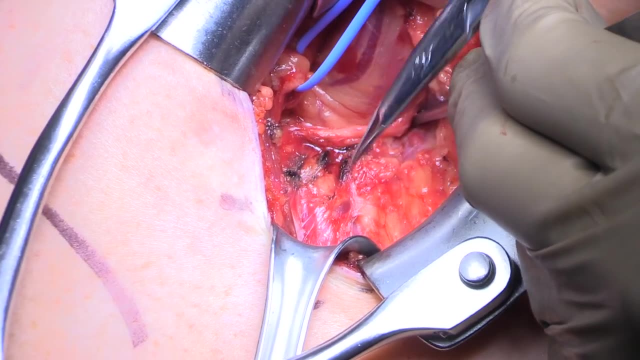 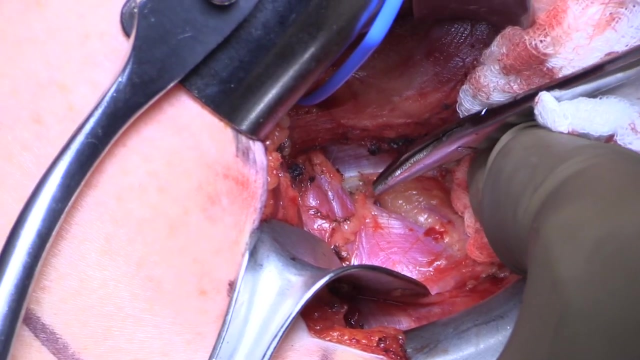 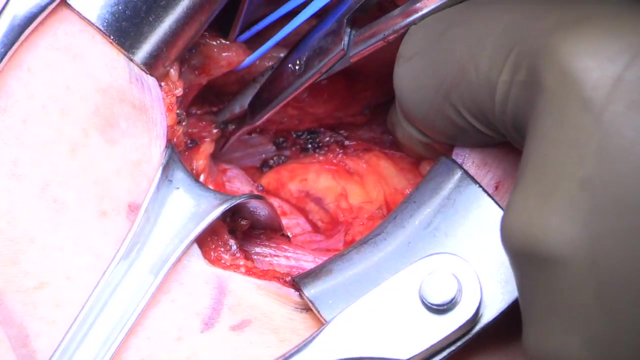 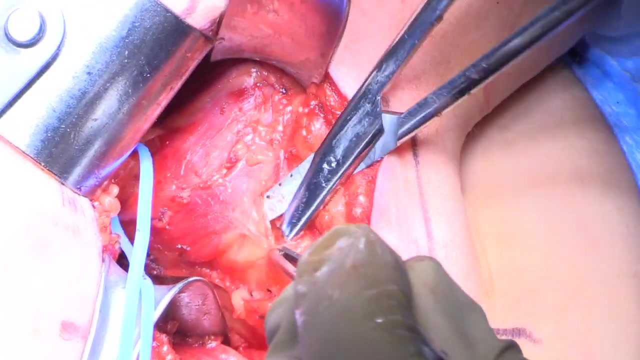 trunk. Further dissection is carried towards the quadrilateral space. Fascial bands are released to decompress the quadrilateral space. Here the surgeon is seen releasing the tight fascial band of the triceps muscle, Although the triceps is not supplied by the axillary nerve. 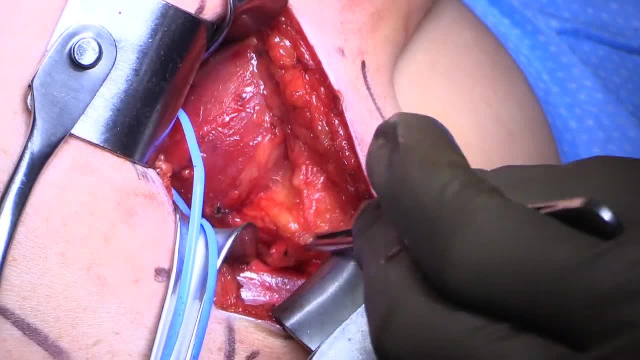 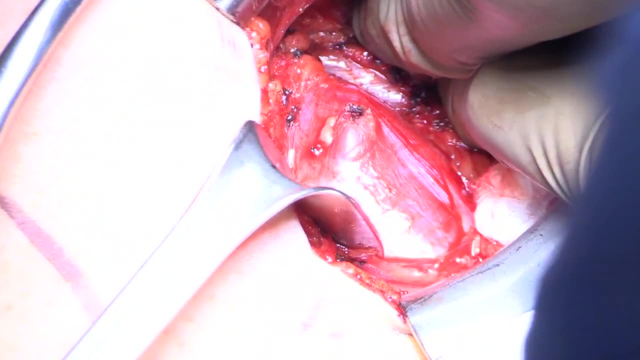 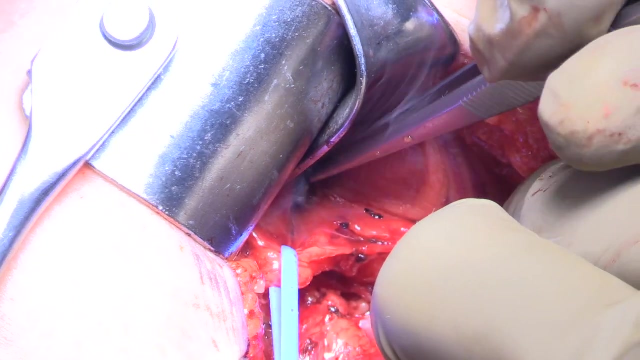 these tight bands can contribute to the compression. It is critical to be mindful during the deep dissection to avoid injuring the posterior circumflex vessels, because they bleed profusely and can retract back, resulting in significant difficulties achieving hemostasis. The surgeon is utilizing an index finger to retract and protect. 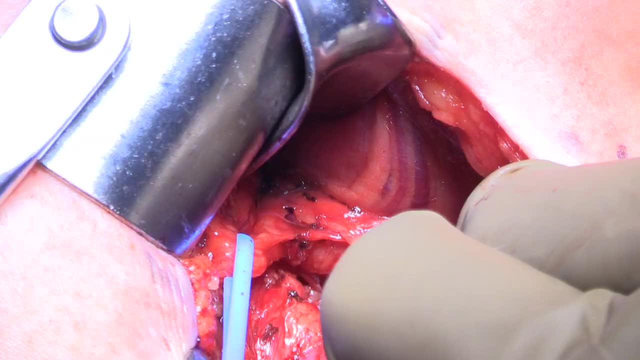 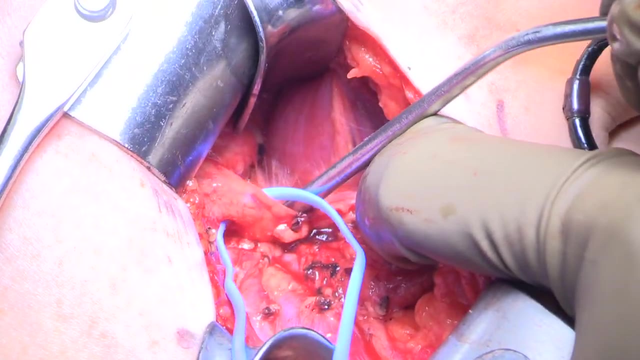 the vessels. Bipolar cautery and peanut dissection is also utilized here. Following this release of the fascial bands, the surgeon achieved a thorough decompression of the axillary nerve in the quadrilateral space and of the posterior humeral circumflex artery. 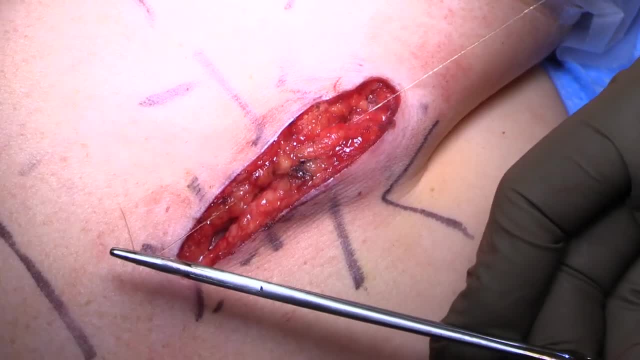 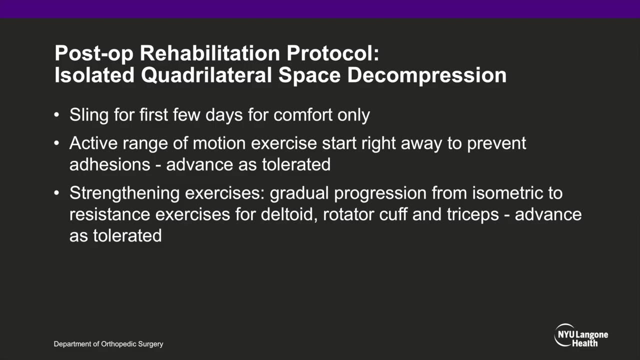 The wound was then copiously irrigated and closed with 3-oh monocryl. Following closure, an arthroscopic labor repair was performed. Because the patient in this clinical case presentation underwent a concomitant labor repair, he required additional range of motion. The patient was then placed in the hospital for a 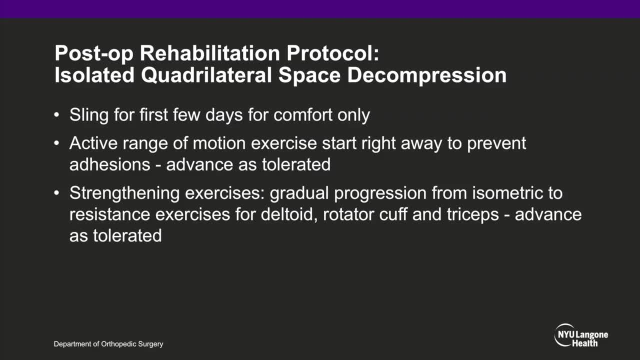 short period of time with additional range of motion limitations. However, in patients undergoing isolated quadrilateral space decompression, the postoperative rehab protocol should include sling for the first few days for comfort, only followed closely by active range of motion exercises to prevent adhesions. 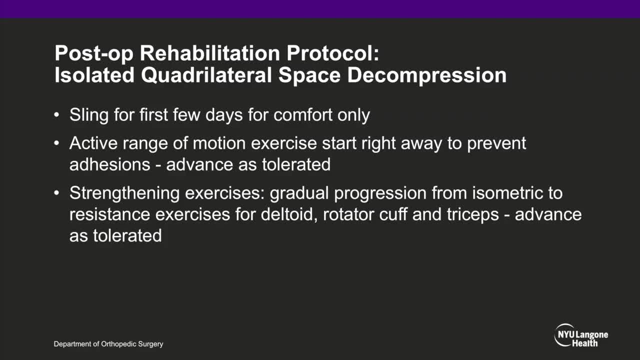 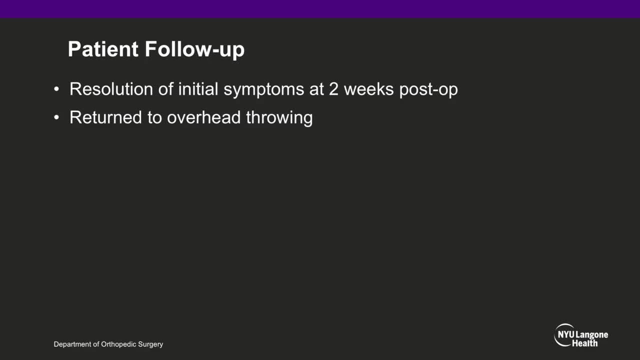 Then the patient should begin strengthening exercises, with a gradual progression from isometric to resistance exercises for the deltoid, rotator cuff and triceps. The patient was seen again at the first post-op visit after two weeks, After two weeks, with resolution of his initial symptoms. and ultimately he returned to overhead throwing.